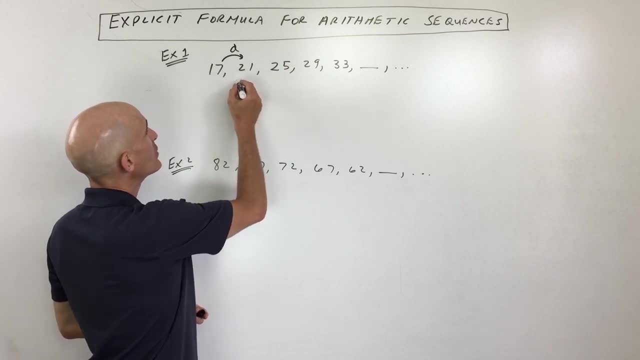 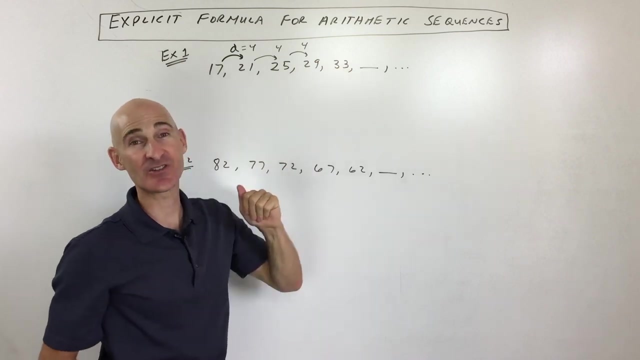 Difference means subtract. If you take 21 minus 17, what do you get? 4. If you take 25 minus 21, what are you getting? 4. If you take 29 minus 25, what are you getting? 4. So what you can see is that common difference is actually what we're adding to get to the next term in the list or in the sequence. So that's why they call it D 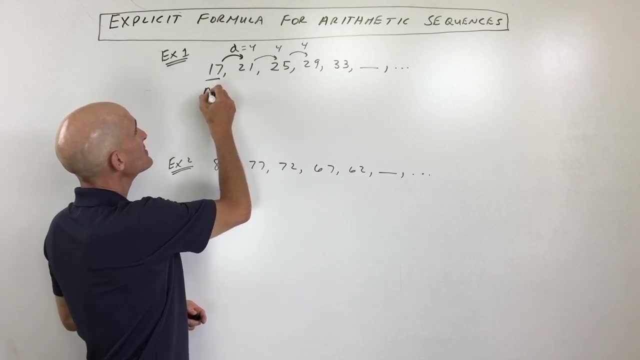 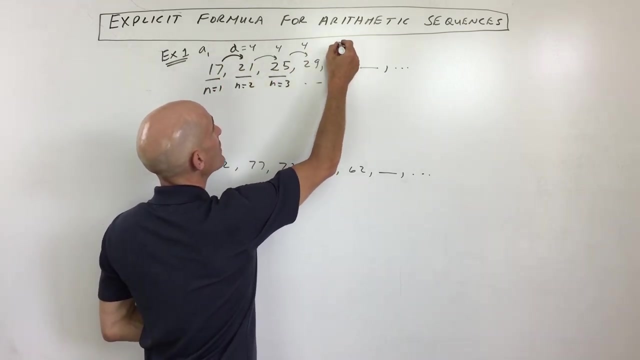 for difference. Now, the next thing I wanted to mention to you is that this is actually called N equals 1, N equals 2, N equals 3, and so on. This means this is the first term, second term, third term. Now, another notation that you want to pay attention to is like A sub 1, A sub 2, A sub 3, A sub 4. Let's write 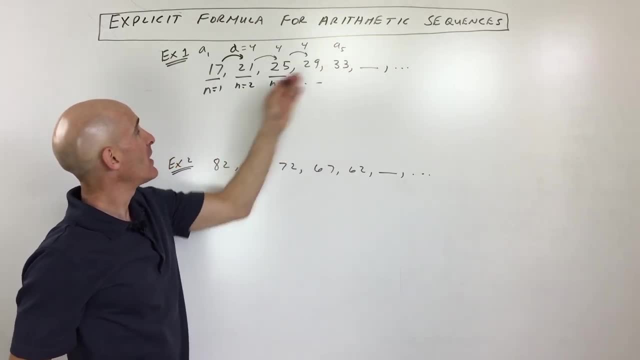 over here A sub 5. That means the value of the fifth term. N is the term number that you're on, but A sub N is the value of that term, what that term actually equals. So now what we want to talk about is how do we find out what 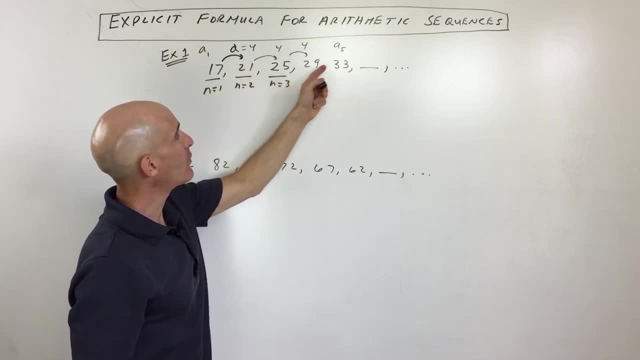 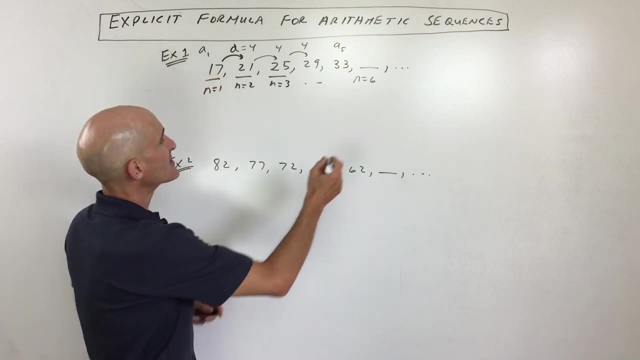 the term is right here? Well, notice this is the 1, 2, 3, 4, 5, 6th term. Okay, so I'm just going to write N equals 6. How do we get to the 6th term? Well, you start off at 17, right? And then what you do is you add 4. Now, how many times are we adding 4? Well, we're adding 4. Once, twice, 3 times, 4 times, 5 times. 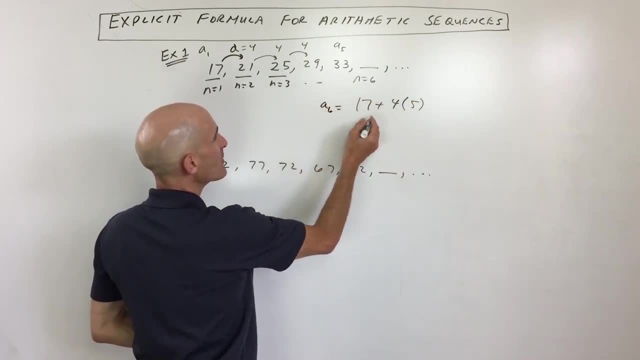 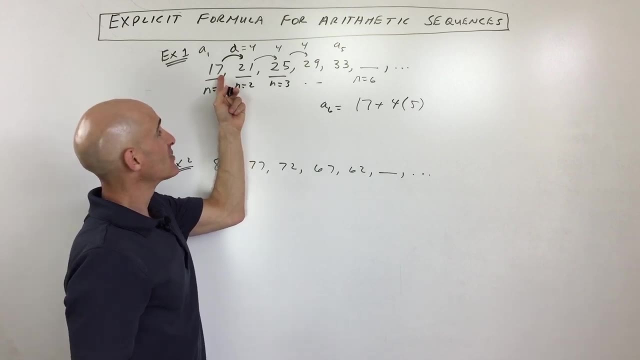 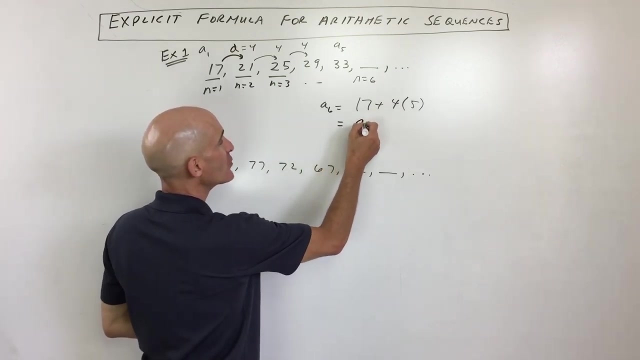 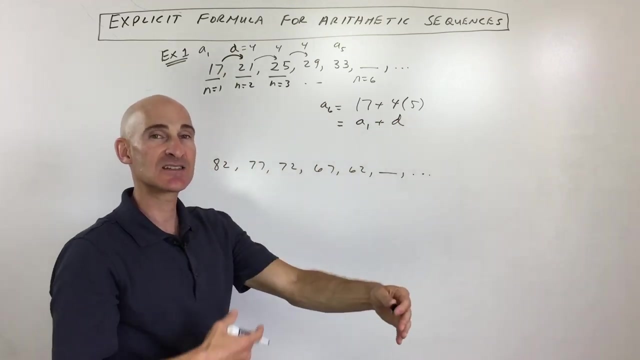 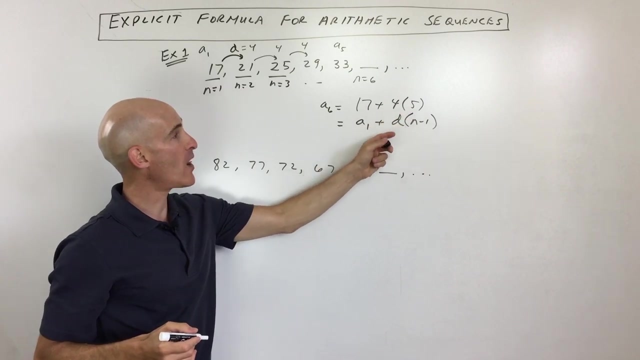 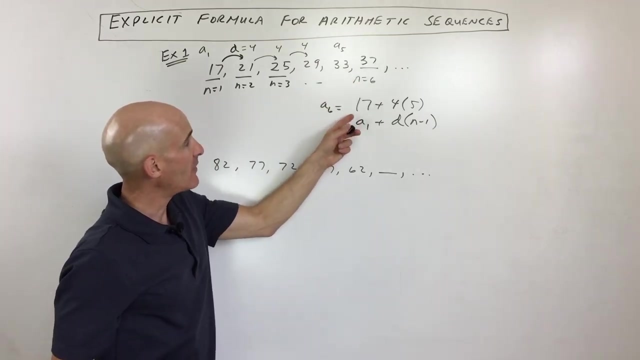 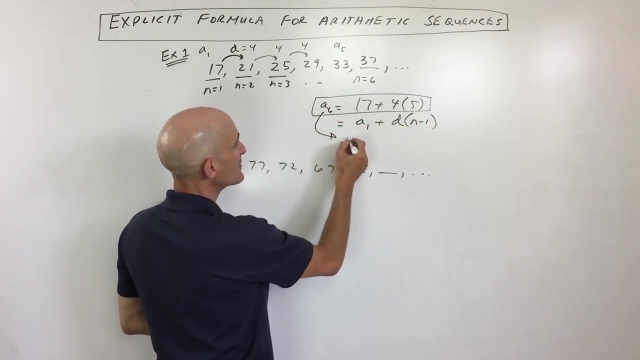 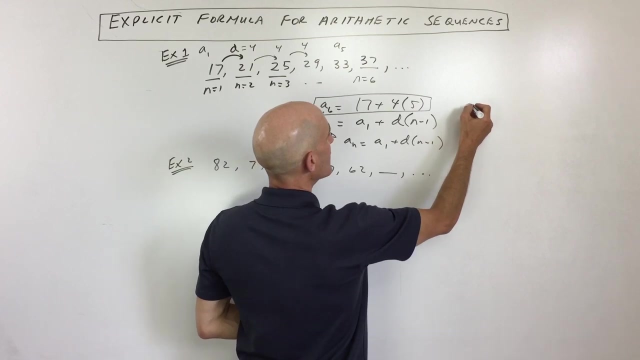 And a lot of students, they'll say, hmm, you found the 6th term, but you added 4 5 times. How come not 6 times, you know? Well, the thing is we're already on the first term. So to get to the 6th term, we only have to add 4 one less time. Okay, so if we wanted to generalize this a little bit more, you could say, well, this is A sub 1. That's the value of the first term. That's 17 plus D. That's the common difference. That's what we're adding to get to the next term. You want to add that D N minus 1 times. Okay, so in this case, you're adding 4 5 times. That's 20 plus 17. That's 37, which makes sense because we were adding 4 each time. So now what we have is we have what they call an explicit formula, meaning that it'll take you right to any particular term. So let's write this in a little bit more general way. A sub N equals A sub 1 plus D times N minus 1. So for this problem, we had, let's see, we had A sub N equals 17. That's the first term. 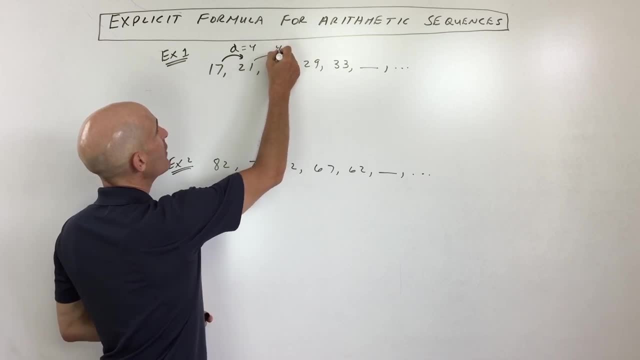 4. If you take 25 minus 21,, what are you getting? 4.. If you take 29 minus 25, what are you getting? 4.. So what you can see is that common difference is actually what we're adding to get to the 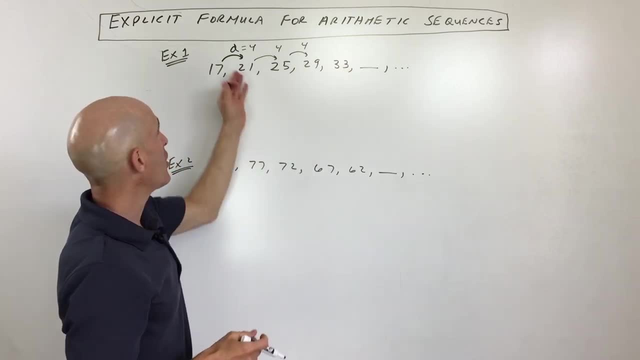 next term in the list or in the sequence. So that's why they call it D for difference. Now, the next thing I wanted to mention to you is that this is actually called N equals 1,, N equals 2,, N equals 3, and so 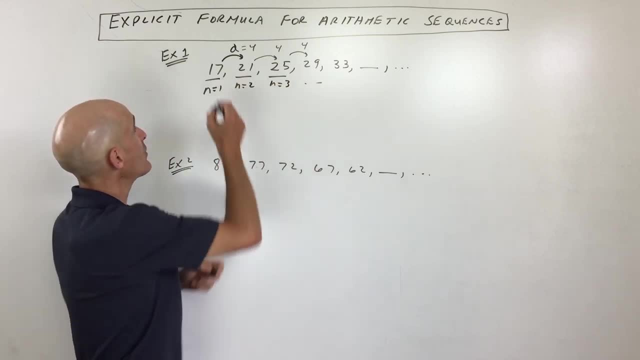 on. This means this is the first term, second term, third term. Now, another notation that you want to pay attention to is like: A sub 1, A sub 2, A sub 3, A sub 4.. Let's write. 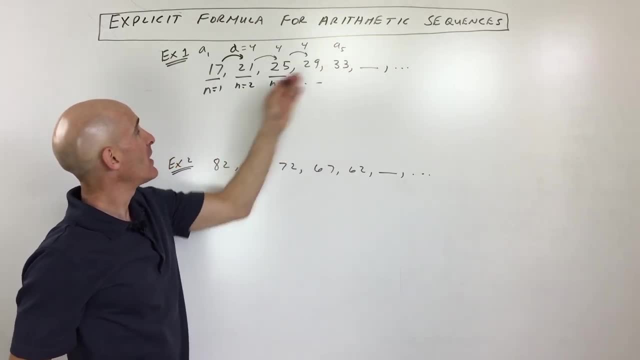 over here, A sub 5.. That means the value of the fifth term. N is the term number that you're on, but A sub N is the value of that term, what that term actually equals. So now, what we want to talk about is: how do we find out what? 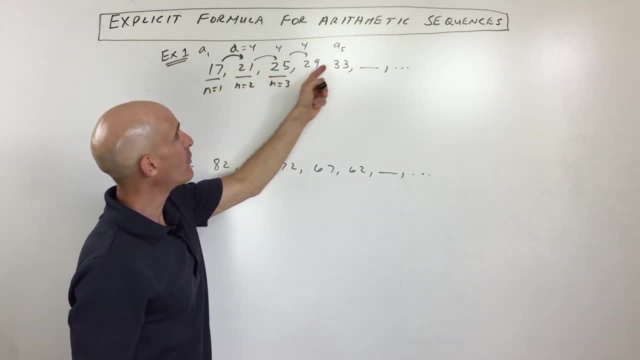 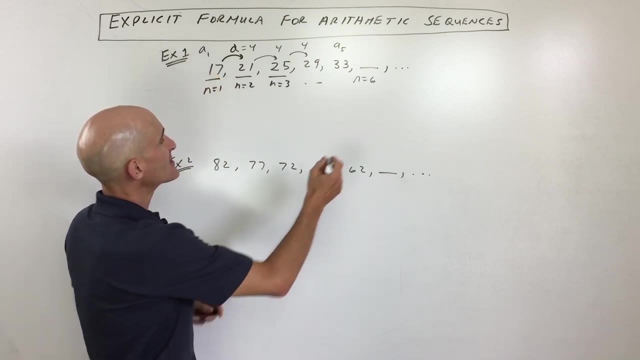 the term is right here. Well notice, this is the 1,, 2,, 3,, 4,, 5, 6th term. Okay, so I'm just going to write: N equals 6.. How do we get to the 6th term? Well, you start off at 17,. 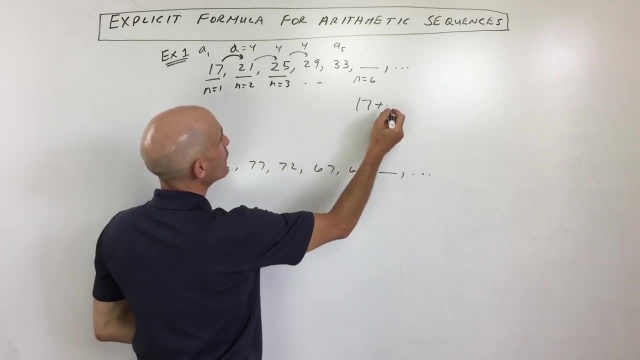 right, And then what you do is you add 4.. Now, how many times are we adding 4?? Well, we're adding 4.. Once, twice, 3 times, 4 times, 5 times, And a lot of students they'll say, hmm, you found the 6th term, but you 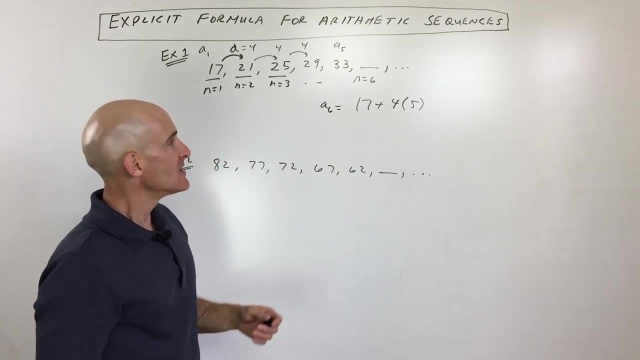 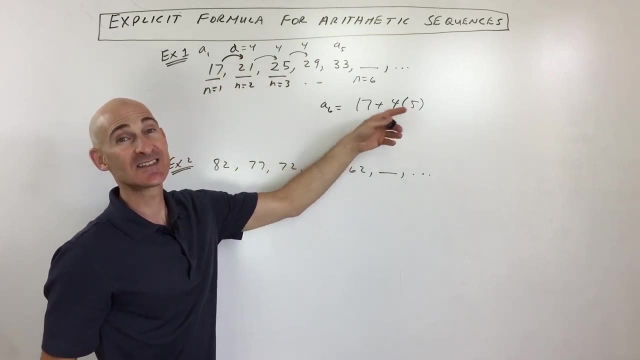 added 4, 5 times. How come not 6 times? you know. Well, the thing is, we're already on the first term, So to get to the 6th term, we only have to add 4, one less time. Okay, so if we wanted, 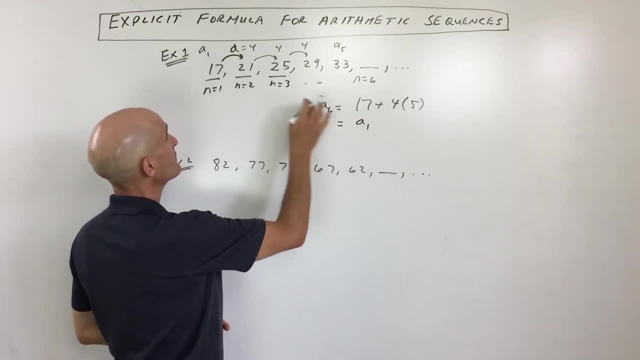 to generalize this a little bit more, you could say: well, this is A sub 1.. That's the value of the first term. That's 17 plus D. That's the common difference. That's what we're adding to get to the next term. 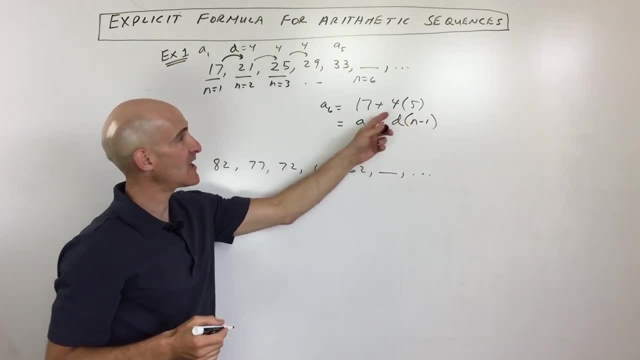 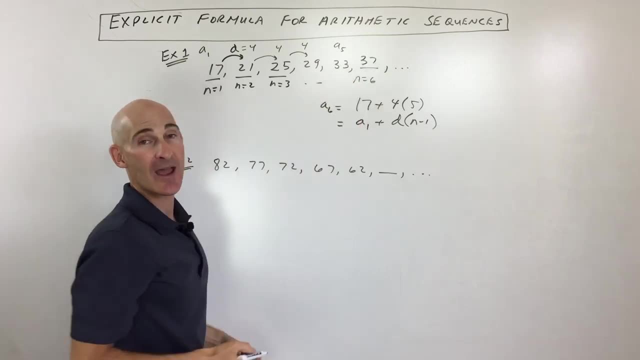 And you want to add that D N minus 1 times. Okay, so in this case you're adding 4 5 times. That's 20 plus 17.. That's 37, which makes sense because we were adding 4 each time. So now what we have. 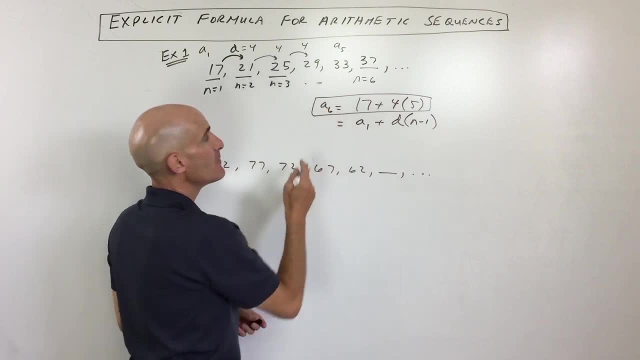 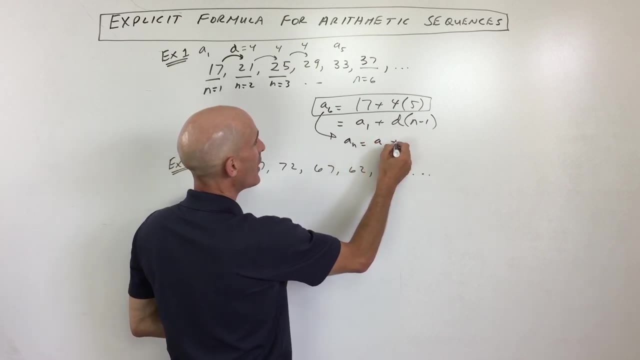 is, we have what they call an explicit formula, meaning that it'll take you right to any particular term. So let's write this in a little bit more general way: A sub N equals A sub 1 plus D times N minus 1.. So for this problem we had, let's see, we had A sub N.